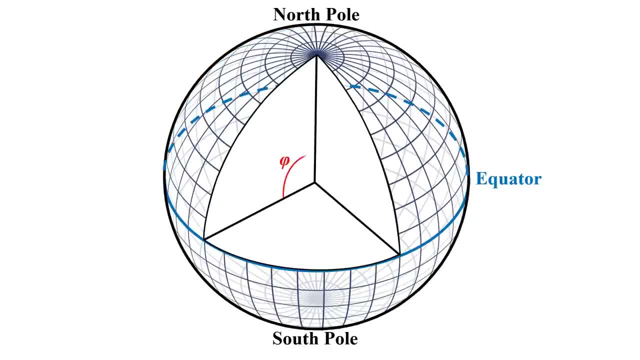 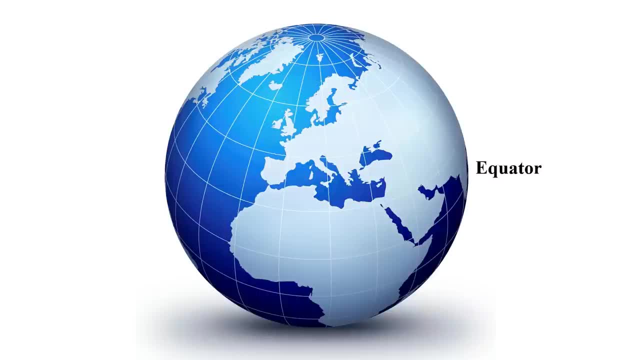 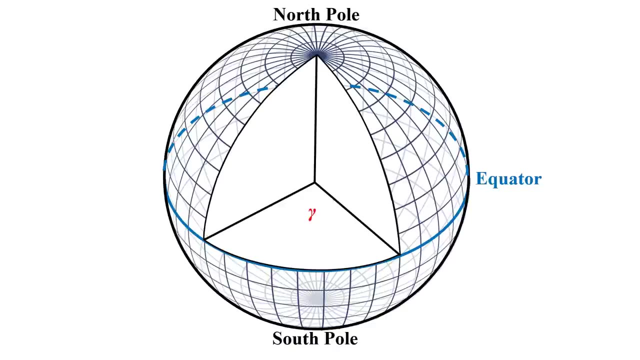 Latitude marked as phi in this illustration is the angle from the equator to the poles. from 0 to 90 degrees north or south from the equator Latitude, lines run parallel to the equator. Longitude marked as gamma in this illustration is the angle from the prime meridian. 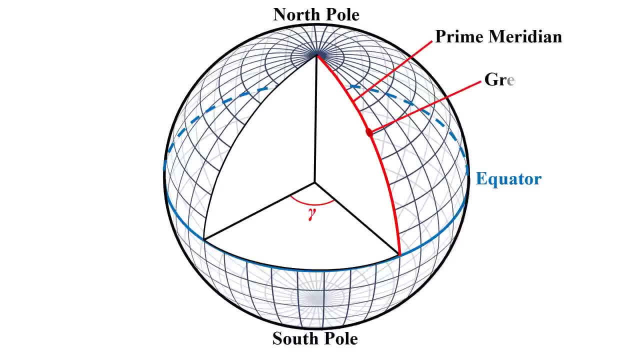 which runs through the Royal Observatory in Greenwich, England. Longitude is the angular measure on the terrestrial sphere, 180 degrees west or east of the prime meridian. Latitude and longitude are both the same. They are both measured in degrees, arcminutes and arcseconds. 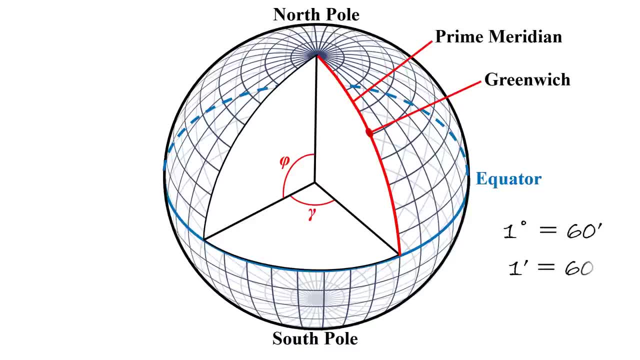 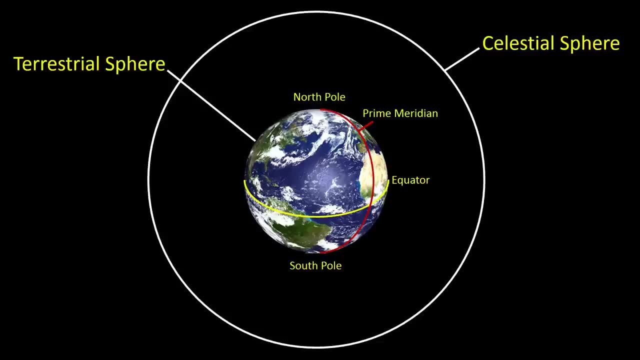 where 1 degree equals 60 arcminutes and 1 arcminute equals 60 arcseconds. There is also a coordinate system for the celestial sphere similar to geographic latitude and longitude. Every point in the celestial sphere maps to one point on the terrestrial sphere. 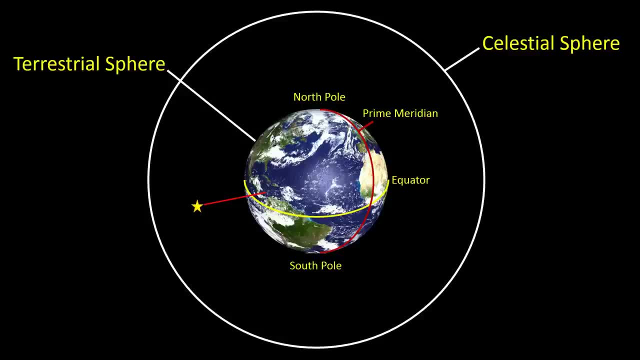 but due to the rotation of the Earth and the motion of the Sun, Moon and planets, these points move in time. In navigation, the celestial coordinate system uses Greenwich hour angle and declination to describe these positions in the celestial sphere. There is a celestial equator which maps to the equator of the Earth. 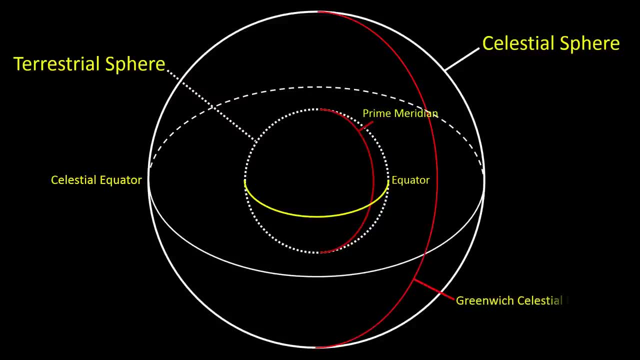 There is also a Greenwich celestial meridian which maps to the terrestrial prime meridian. Greenwich hour angle, abbreviated GHA, is an angular measure along the celestial equator westward from the Greenwich celestial meridian, similar to longitude Declination. abbreviated DEC. 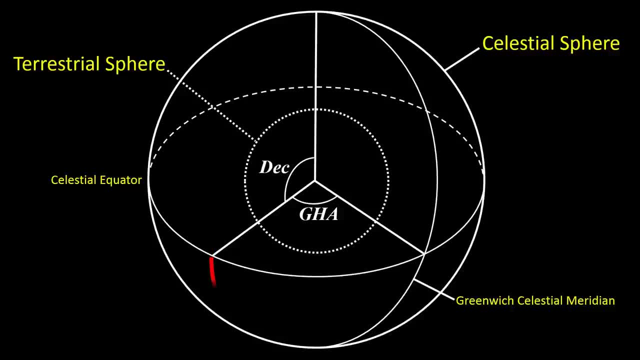 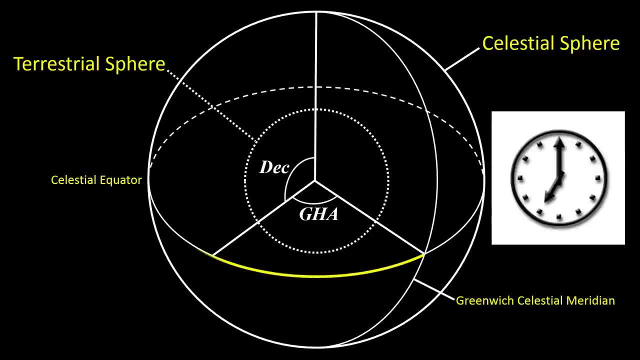 is an angular measure north or south from the celestial equator, similar to latitude. GHA can be measured in degrees or in time, where 24 hours equals 360 degrees, hence the term hour angle. In navigation, both GHA and declination are measured in degrees, arcminutes and arcseconds. 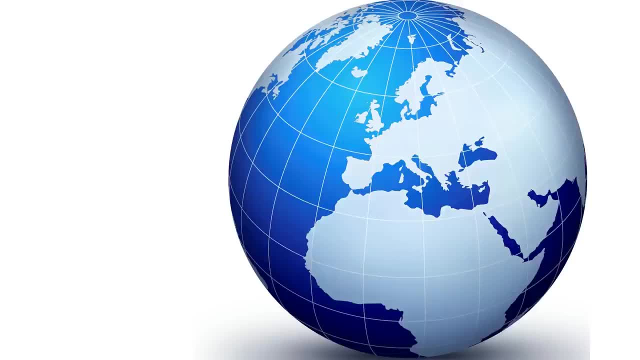 At any given moment, every celestial body may be mapped to the Earth, as there is one point in the terrestrial sphere where the celestial body lies directly overhead. This is called the celestial body's geographic position, or GP. If you were standing at the geographic position,